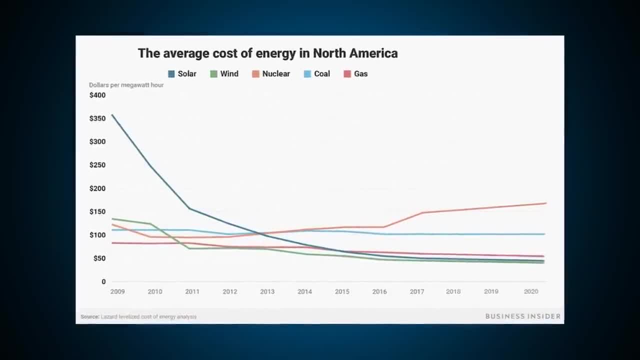 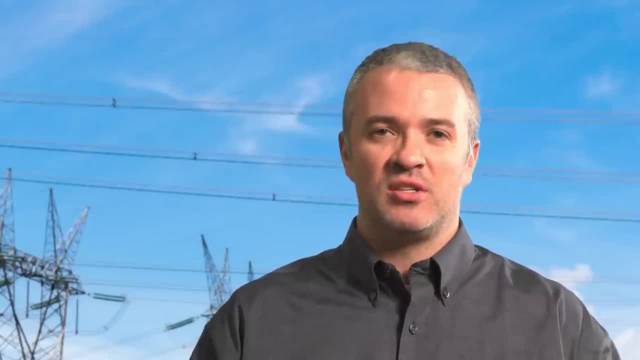 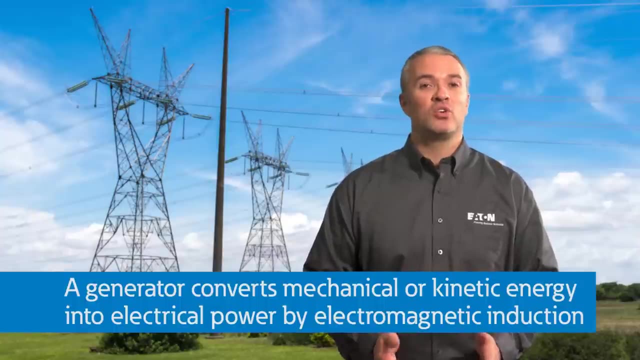 This is changing as renewables and natural gas are becoming more cost effective. Utilities produce this energy inside of large power plants, also known as generation stations. Let's start with the question: what is a generator and how does it work? A generator converts mechanical or kinetic energy into electrical power or electricity. 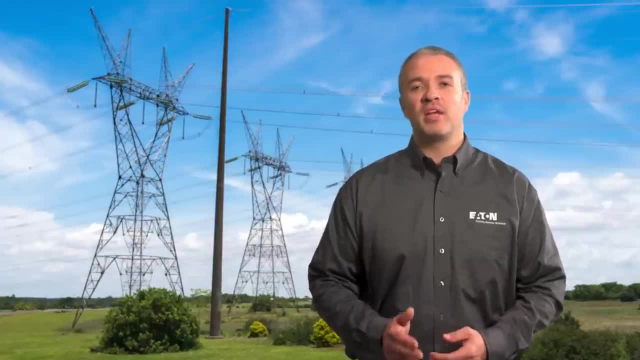 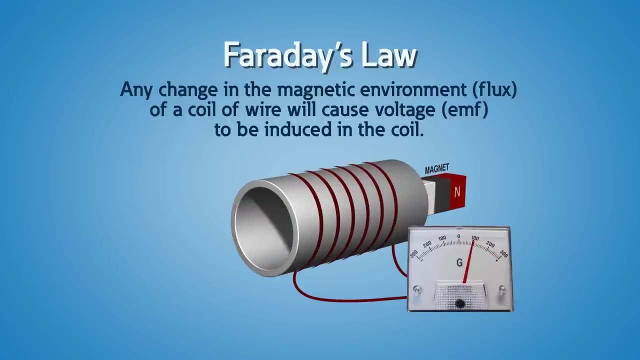 by electromagnetic induction, which is simply varying a magnetic field within a coil of wire. This phenomenon is explained by Faraday's Law, as shown here in this example. As that induced current travels in a loop on the wire, it will create a current that will 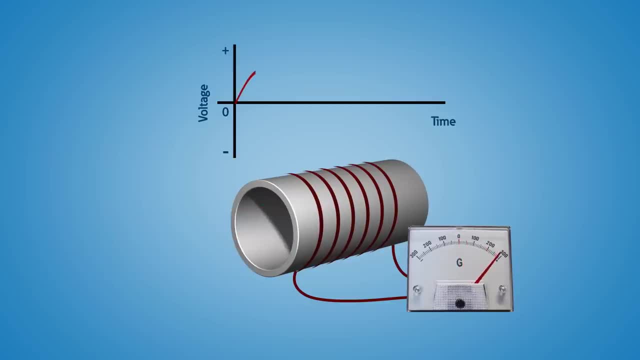 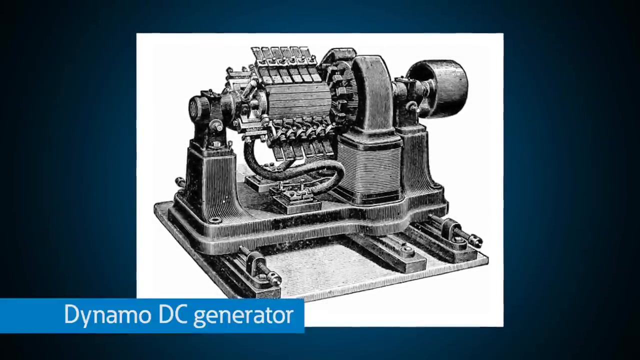 create a magnetic field. Because the field is continuously changing or alternating, it creates what we would call a sine wave or alternating current waveform. Historically, the first generator invented was a direct current or DC generator called a dynamo DC. power produced by these generators was limited because the generation source 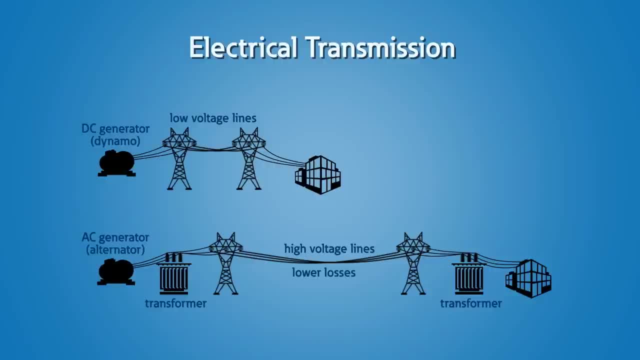 had to be close to the loads. Then came alternating current produced by AC generators called an alternator or a synchronous generator. The major advantage of the AC generation is that with transformers the voltage levels can be changed up and down to transmit that power far distances to the loads that require it. 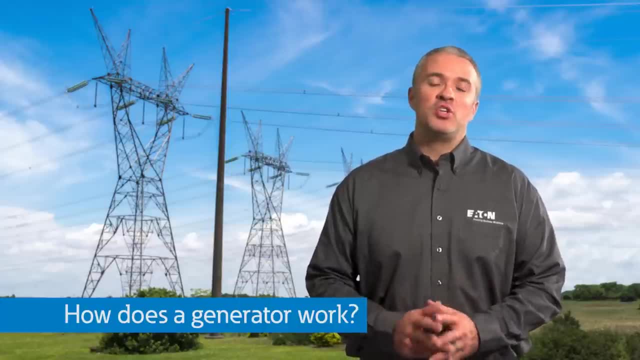 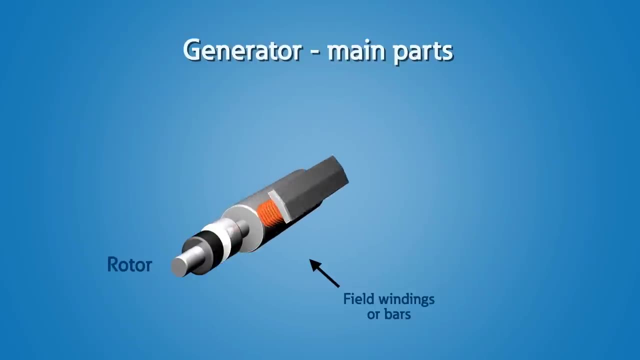 So how does a generator work? The two main parts of a generator are the rotor and the stator. The rotor is the part that rotates and consists of many loops of copper wire or bars called field windings. Field windings are used to create the magnetic field induced. 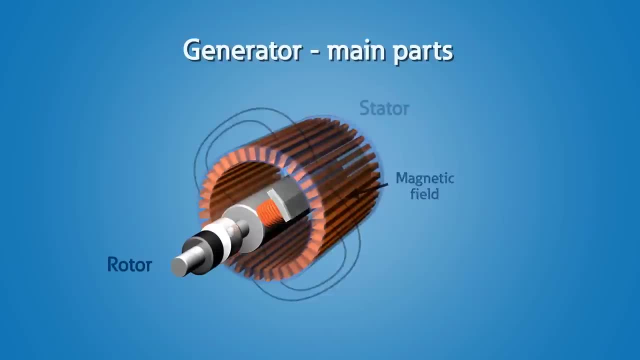 on the metal core to which the wire is wrapped around. The stator is the stationary or static part of the generator that consists of copper windings called armature windings. The power that is produced by the generator will flow out of these armature windings towards the load. 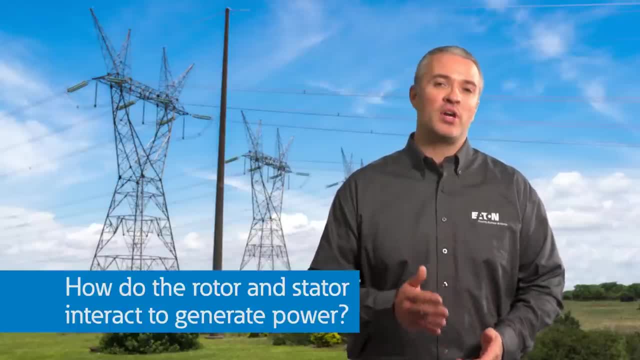 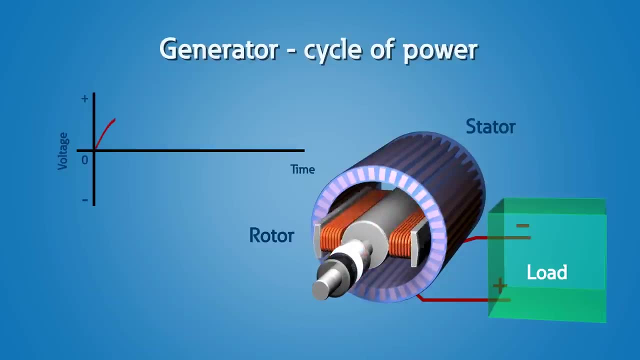 Let's get a better understanding of the basics of how the rotor and stator interact to generate power. First of all, we need to understand that the rotor spins inside the stator and one full rotation is equal to one full rotation In North America. this would equate to one 60 Hz cycle For a generator to produce power. 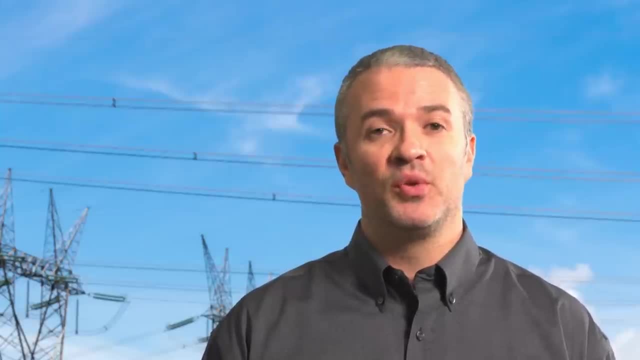 an electromagnetic induction must occur between the field windings in the rotor and the armature windings in the stator. A magnetic field must be created in the field windings on the rotor. Traditionally, this was done using permanent magnets, but with larger scale generation being needed. 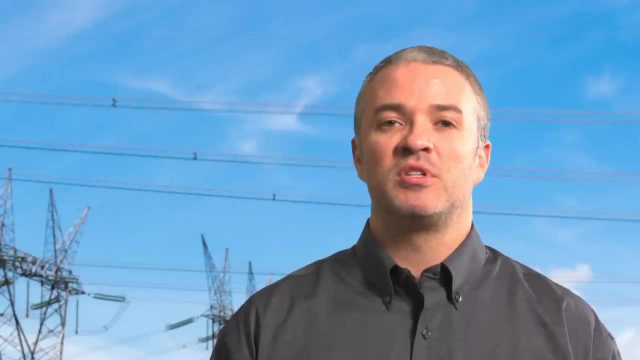 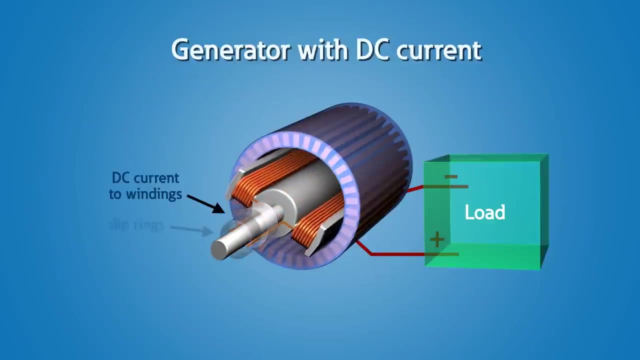 electromagnetic field coils were able to produce substantially more power. This is done by applying a DC current or excitation current to the field windings through a pair of carbon brushes and slip rings. Slip rings are attached to the shaft of the rotor and spin with the rotor while brushes are stationary. 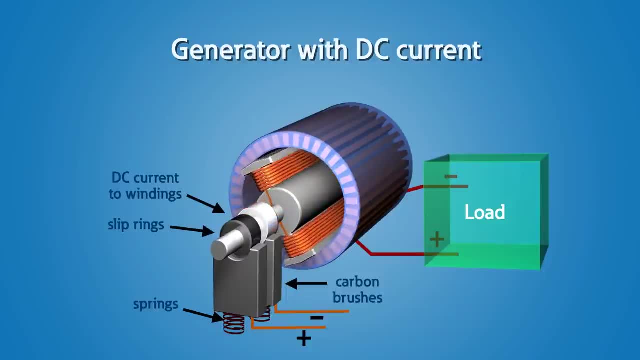 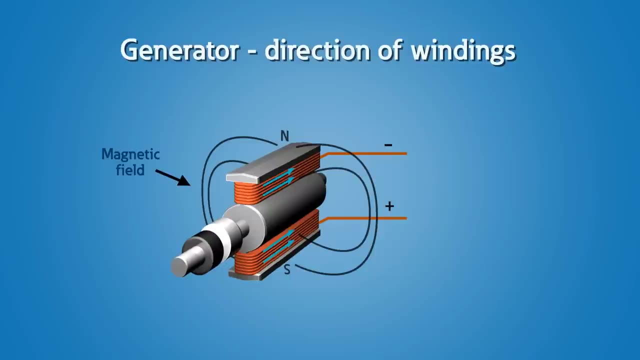 and connect to the end of a wire with a spring pushing on them against the slip ring, making an electrical connection. The field winding is a continuous wire that is looped around a certain number of poles that are part of the rotor core, with positive polarity connected on one end and negative polarity connected on the other. 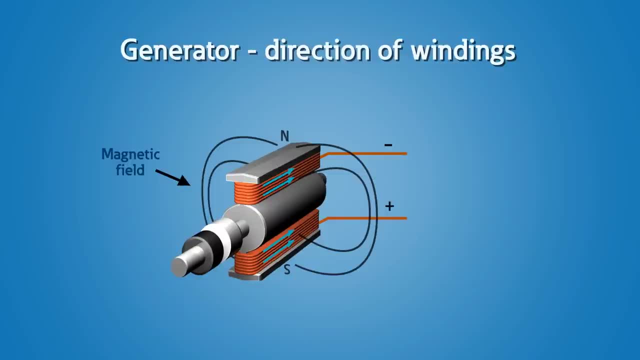 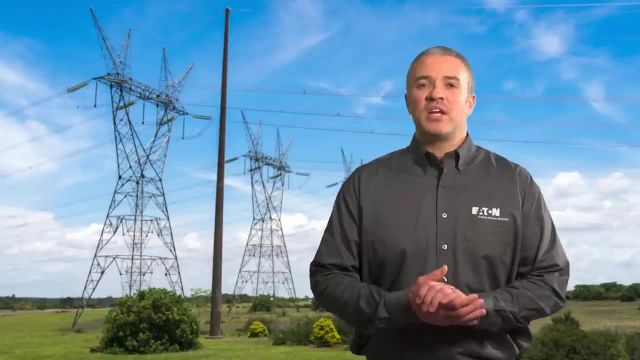 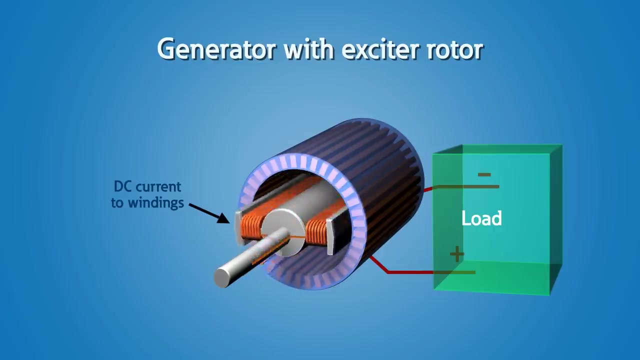 negative. on the other, North and south poles will be created, depending if the coils are wrapped clockwise or counterclockwise around the poles. This essentially is creating an electromagnet with the DC source. This DC current can come from an external source or from a small exciter rotor with a rectifier. 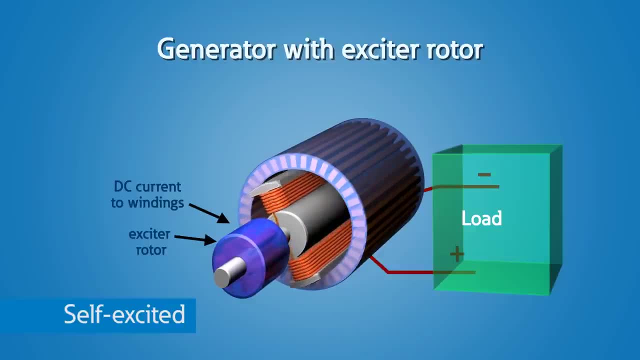 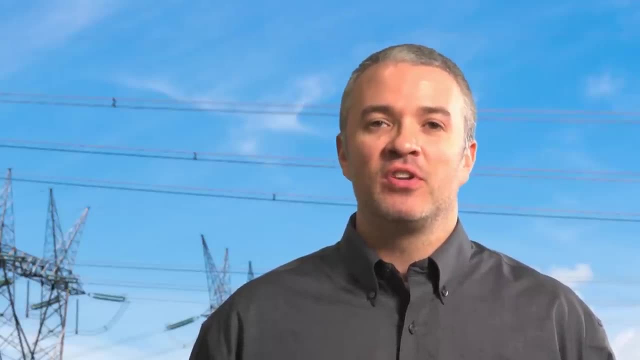 that is attached at the same shaft as the main rotor and is called self excited. This excitation current is a crucial part in the voltage regulation of the generator. The magnetic field strength of the field windings on the rotor can increase or decrease by changing the amount of excitation. 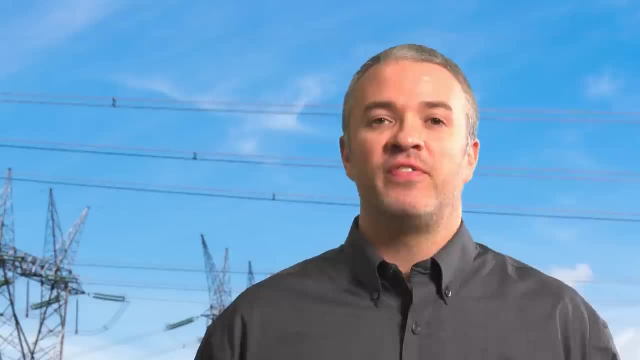 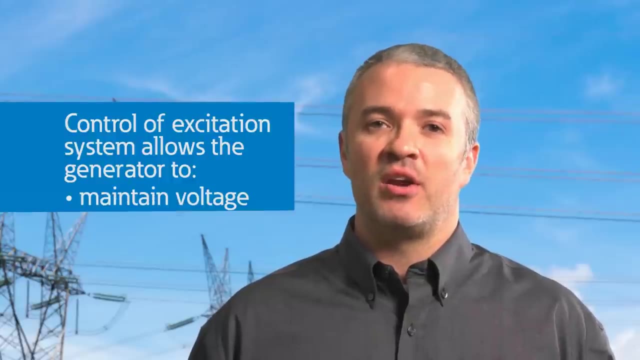 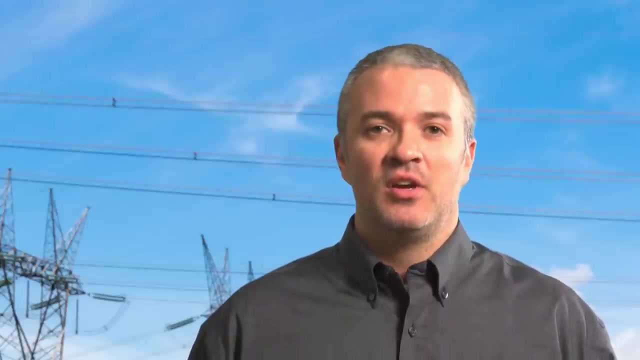 current. The amount of current in the number of turns in the field windings determine the strength of the magnetic field. The control of the excitation system allows the generator to maintain voltage, control reactive power flow and assist in maintaining power system stability During load changes or. 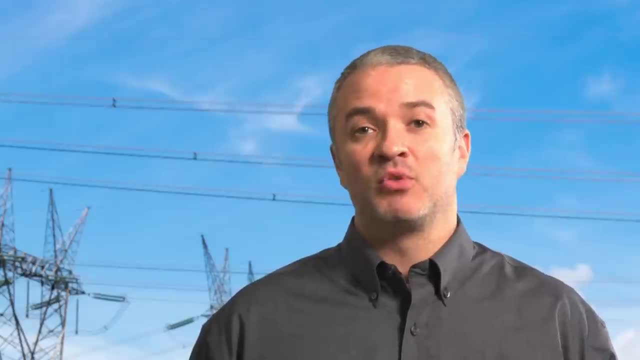 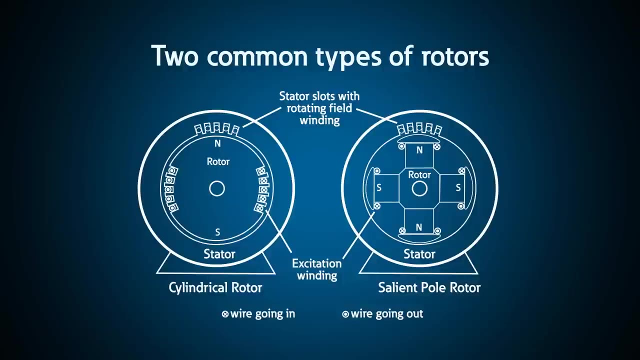 disturbances on the system. the exciter must respond, sometimes in a couple of seconds, to the power supply. The power supply can be rapidly to maintain the proper voltage at the generator terminals for the load. The two common types of rotors are cylindrical and salient. Cylindrical will 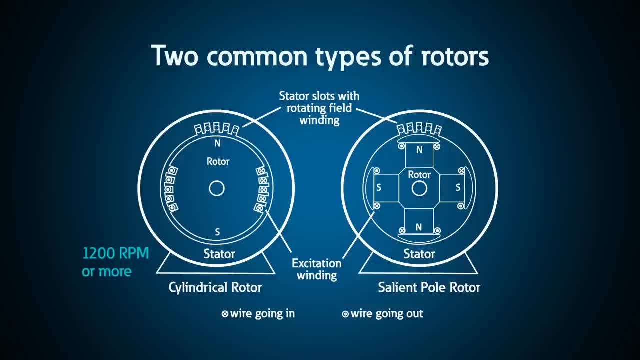 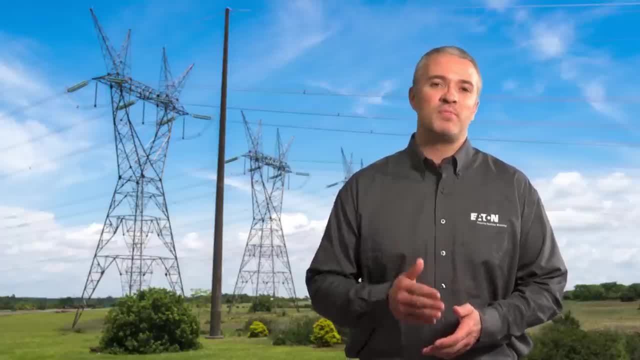 generally operate at speeds of 1200 rpm or more and salient at speeds below 1200 rpm. So we know how the magnetic field is created on the poles of the spinning rotor. now let's see how the field transfers onto the armature windings or 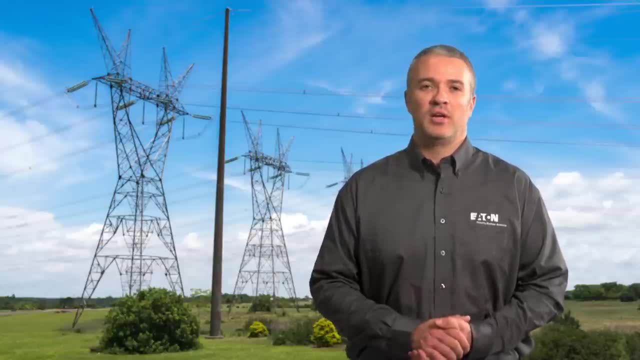 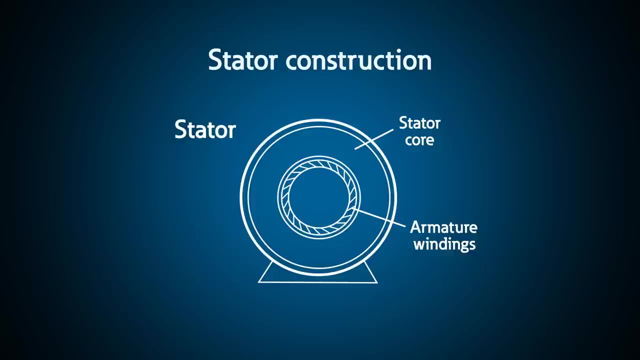 poles of the stator and turns into usable power. The stator is enclosed inside a metal housing and consists of two main parts: The outer part of the stator, called the core, and the armature windings. The core is generally made of a. 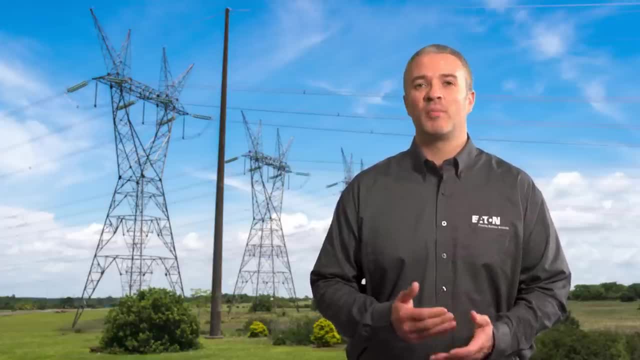 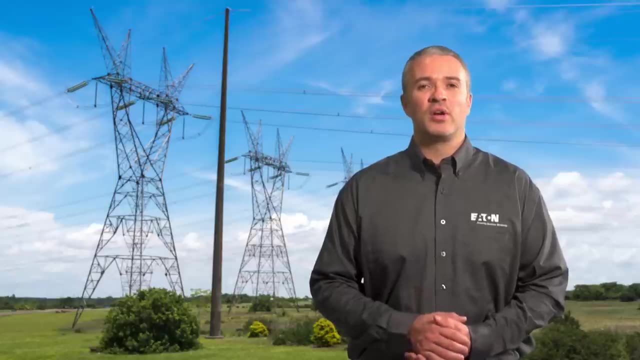 low-loss magnetic material and used to support the coils of the armature windings and is also a return path for the lines of magnetic field. The magnetic field created on the rotor induces a current onto the armature windings. The stator will then transfer to the stator and turn into usable power. The stator. 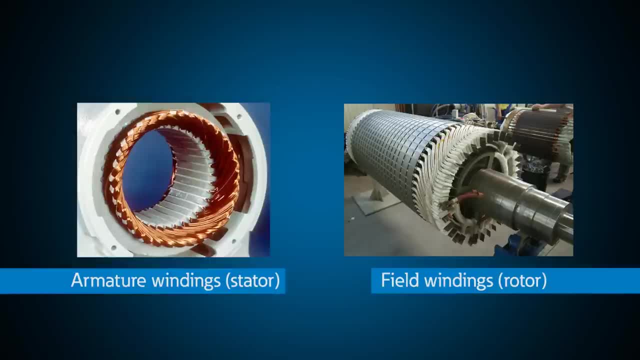 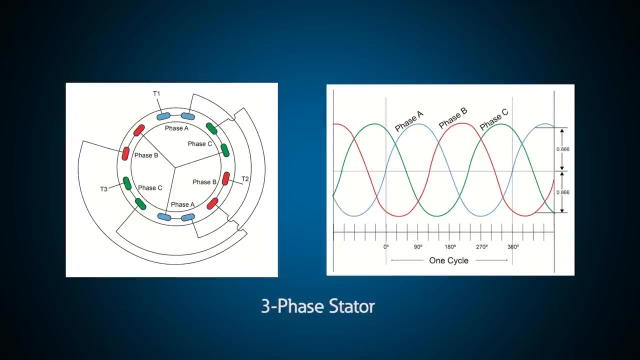 windings tend to be larger, highly insulated and more complex than the field windings in the rotor because they must carry the generated power through them, that is, of a much higher voltage. A three-phase stator will consist of three windings where, for each phase, there is one group for each rotor pole. Each group 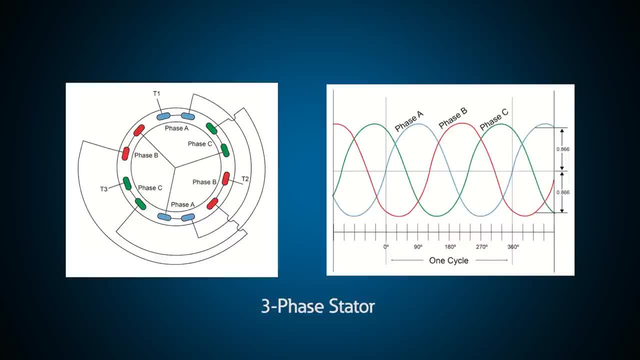 is interconnected and can be considered as one large coil. Each group has an output lead from a generator that is 120 degrees from one another. The leads are typically wide, but the stator has a large output lead that is 120 degrees from one another. The leads are typically 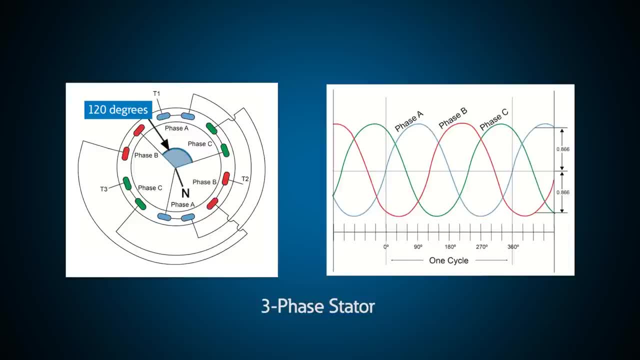 wide or star-connected, and the neutral is usually connected to ground or brought out with single phase loads. As the rotor spins, three separate voltages are created at the stator terminals. There are other considerations in the stator's armature windings to consider, such as how. 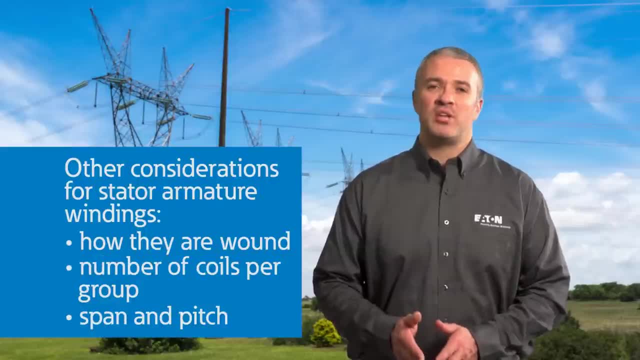 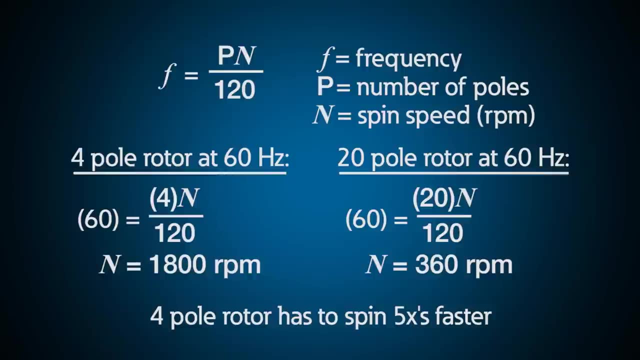 they're wound? how many coils per group? as well as span and pitch, The frequency of a generator is directly related to the number of poles on the rotor in the speed of which it spins. For example, for a four pole rotor posting a rotor with four. 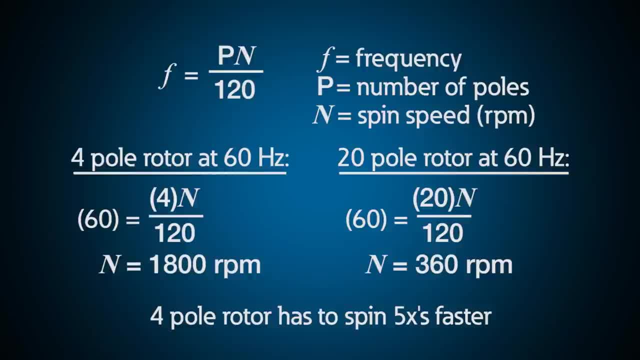 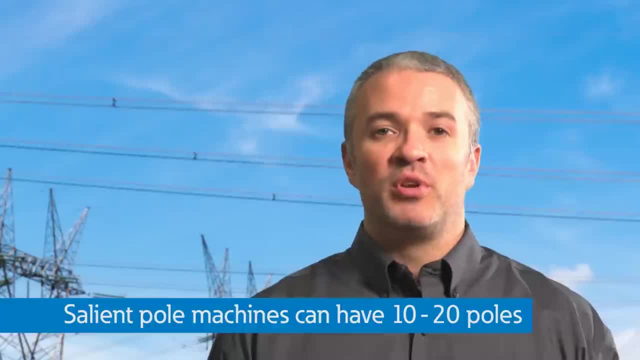 rotor to rotate at 60 hertz, it would have to spin five times faster than a 20-pole rotor, putting much more mechanical stress on the generator. Salient pole machines may have 10 to 20 poles, reducing the stress on these generators. 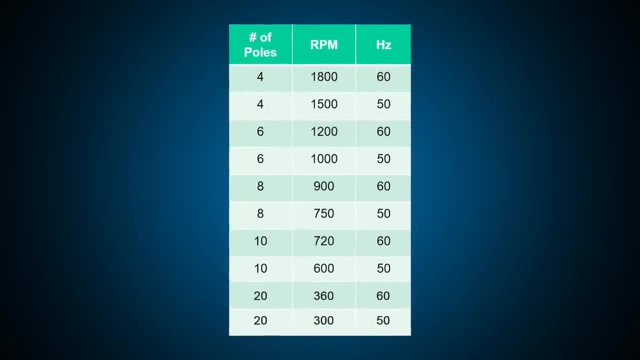 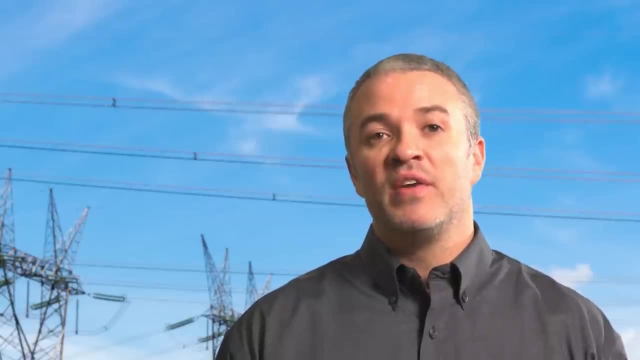 but again run at a lower RPM. Power plants may choose a rotor with a certain number of poles, depending on the speed needed for the application. In other words, if the device that will be spinning the rotor, known as the prime mover, has a certain operating speed, the rotor can be. selected based off of that RPM. Even with large fluctuations in load, large utility generators don't allow the frequency to change much because they are large rotating masses and provide significant inertia to the grid. This is extremely beneficial to the grid by stabilizing the voltage. 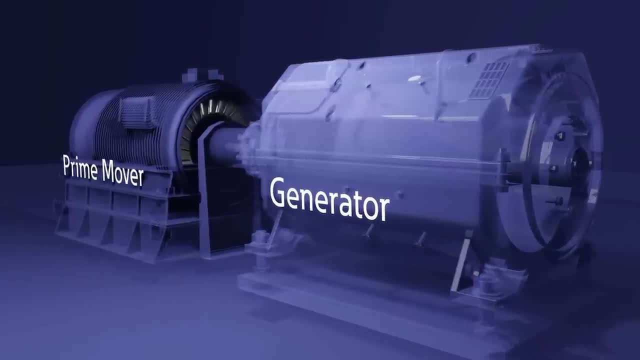 but it could take up to a minute for these units to get frequency back to the proper level if something catastrophic happens, because they are so large. Some want to use the voltage to control the voltage, but they don't want to do that. Some want to use the voltage to control the voltage, but they don't want to do that. 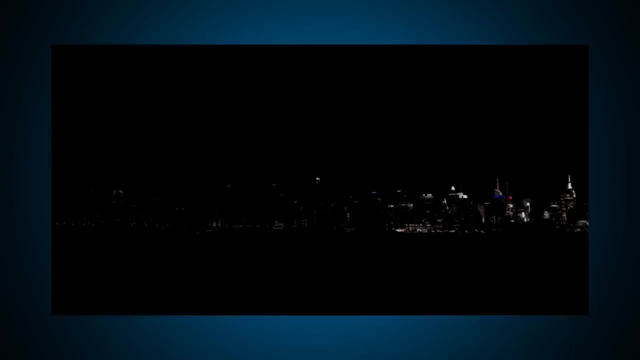 Some want to use the voltage to control the voltage, but they don't want to do that. Widespread blackouts have been related to significant frequency changes in the response of large generators and groups of generators. Wind and solar have a much faster frequency. 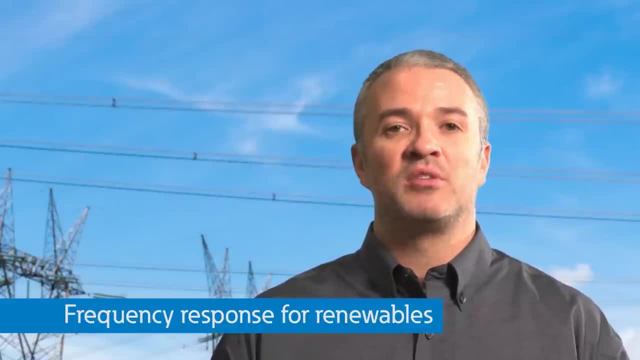 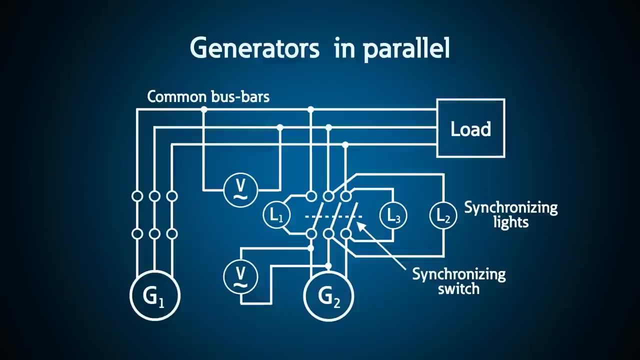 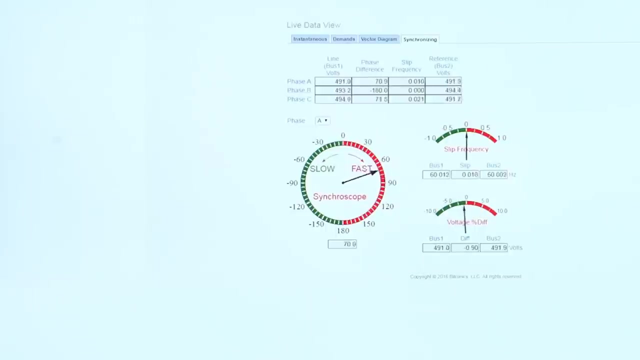 response due to the use of electronics, but they don't provide as much grid stability provided by large generators with rotating inertia. For large systems, generators are paralleled with each other to provide more capacity to feed loads and they must be synchronized with each other. The objective of synchronization is to match speed. 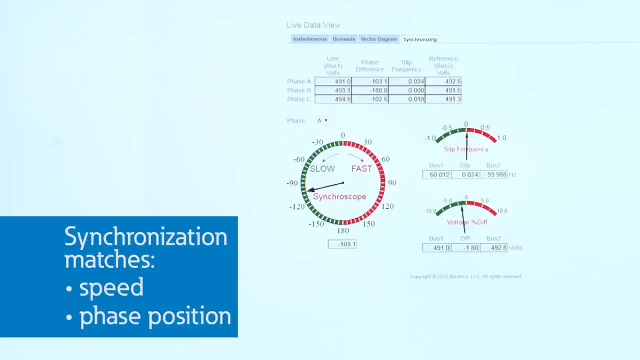 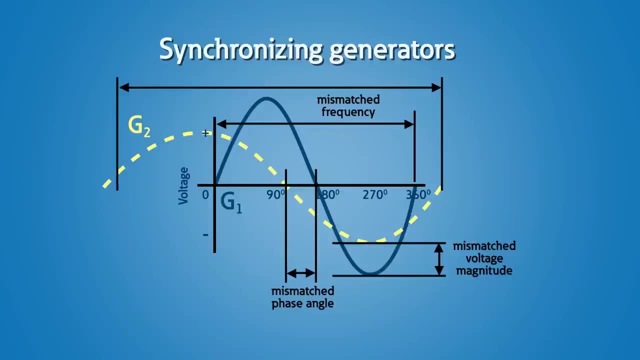 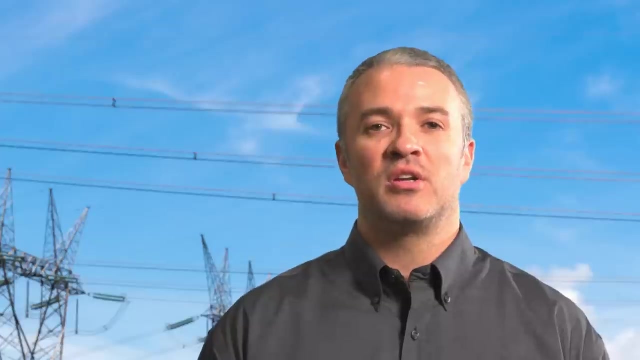 and phase position. so there is little or no transfer of energy when paralleling multiple units or connecting to an existing grid, or bad things could happen. Synchronizing requires matching voltage, magnitudes, frequency and phase angle On systems with commercial or industrial generators. 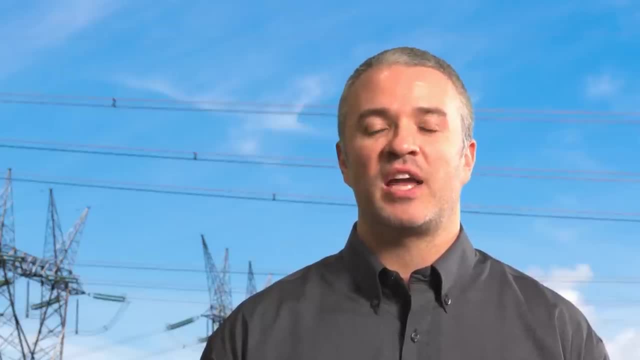 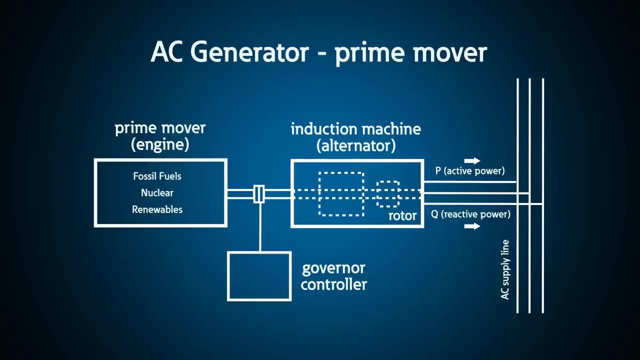 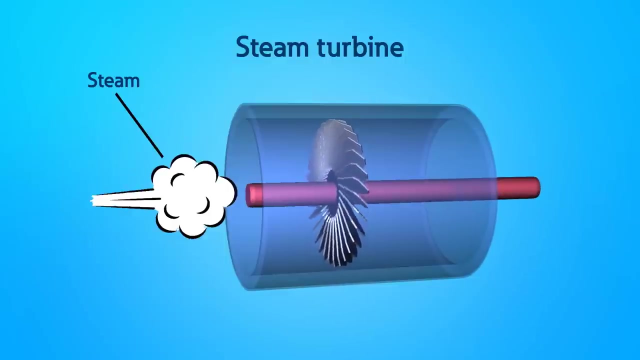 synchronizing these generators requires a special transfer switch with that capability. AC generators have a lot of moving parts, but the main power producing component is the prime mover. The most common prime mover is a steam turbine or turbo machine. It consists of at least 1 moving part. 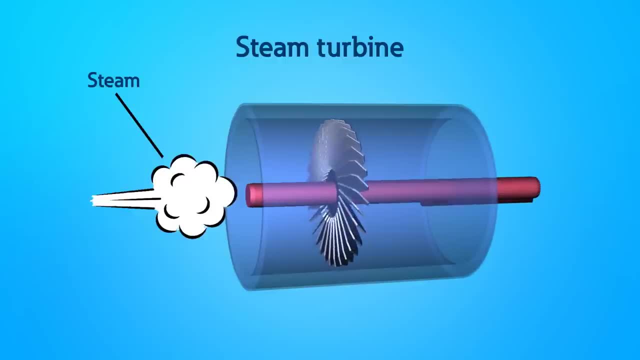 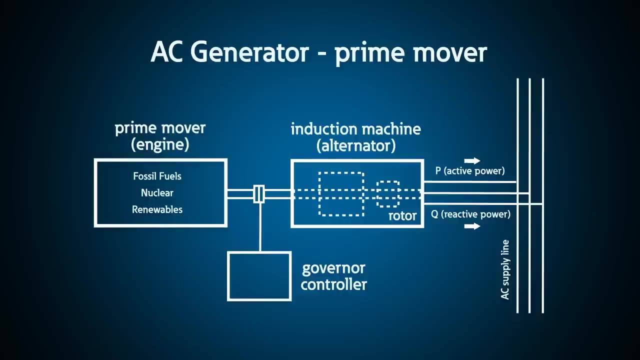 called a rotor assembly, which is a shaft or drum with blades attached and used in thermal power plants. This part makes the rotor spin at the desired speed by using mechanical gears. Governors on the prime mover system are used to control the speed of the prime. 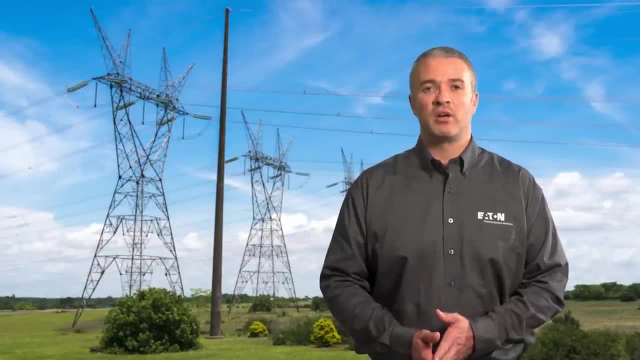 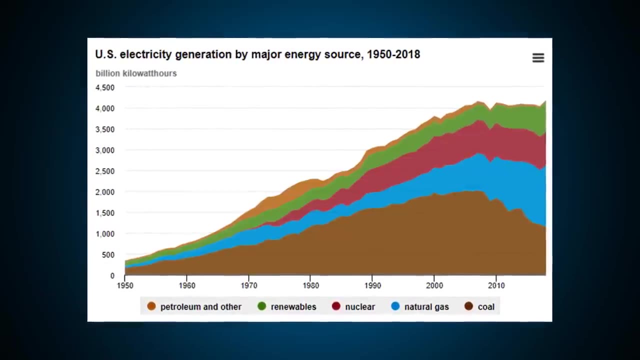 mover, which then that controls the speed of the rotor inside the generator. Most of the generation today is still being produced by the general unreal director or generator. conventional generator Le Filip пред boiler and burning of fossil fuels, with coal being the primary fuel of choice. but in the united states 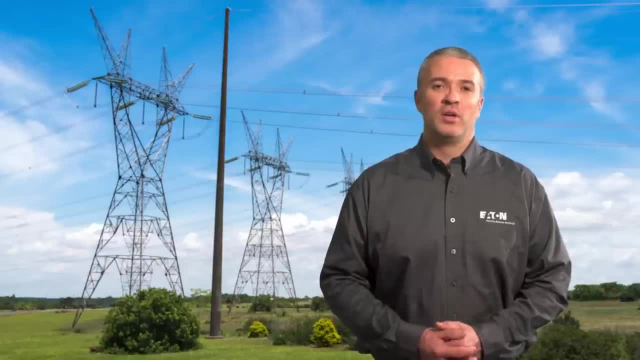 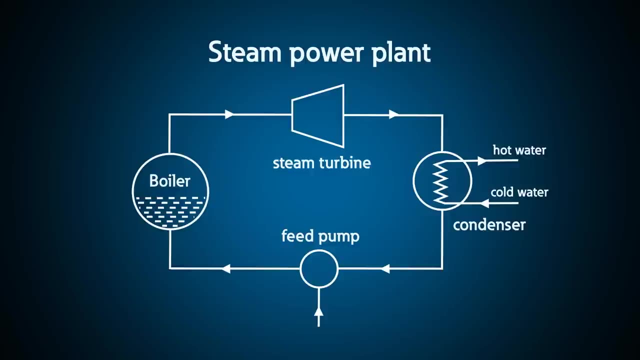 natural gas has recently become the leading fuel over coal. when fossil fuels are burned, they create heat that boils water in a boiler, producing steam, sending it to the condensing turbines, and then exhaust that steam to a condenser. the exhausted steam is the white smoke that you would see coming. 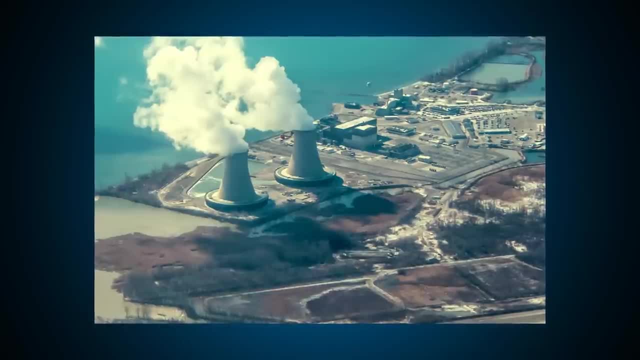 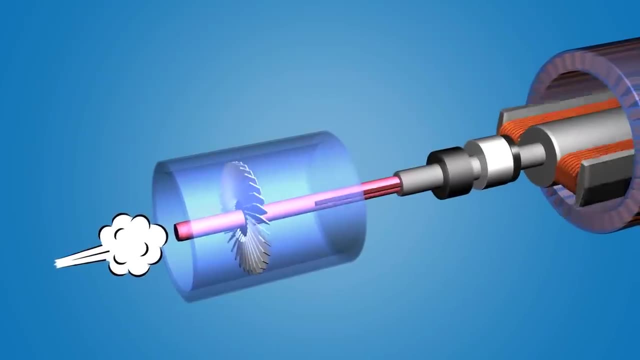 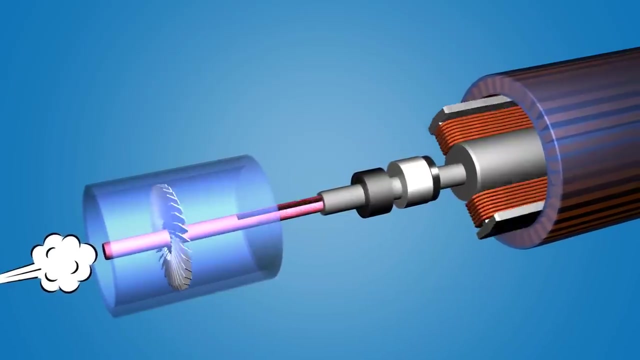 out of cooling towers at a generation station, and it is of no danger to the environment. the steam turbine is a form of heat engine that extracts the thermal energy from the pressurized steam and uses it to do mechanical work on a rotating output shaft. this ultimately spins the rotor of 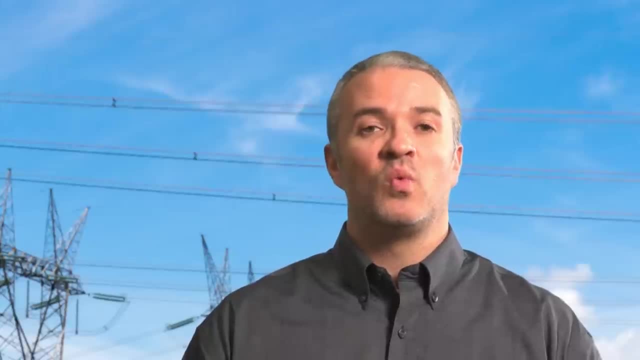 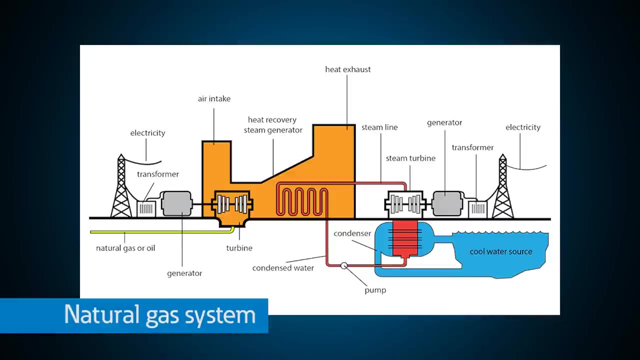 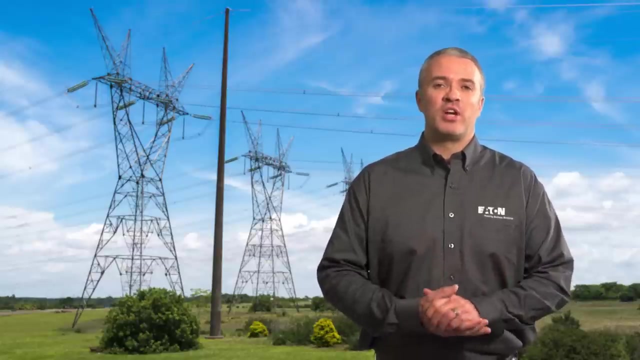 the generator. not all fossil fuels are used to heat water, to produce steam. natural gas power plants can also burn natural gas mixed with a stream of air, which combusts and expands through a gas turbine to spin as its primary mover. nuclear power plants are another type of generation source. 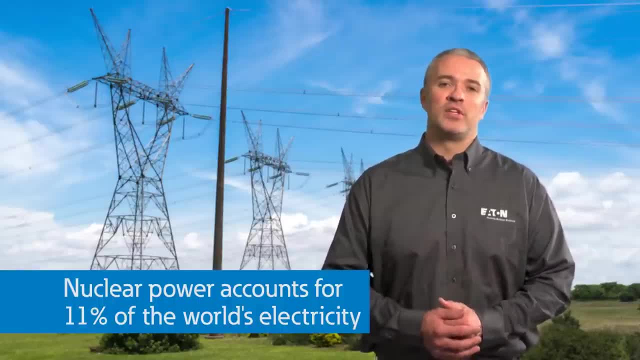 that can be used to produce steam from a steam turbine. the steam turbine is a form of heat engine that extracts the thermal energy from the pressurized steam and uses it to do mechanical work on a. that provides a very large amount of power and about 11 of the world's electricity. in the united 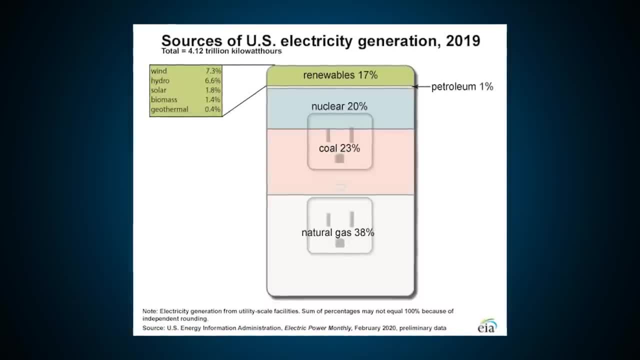 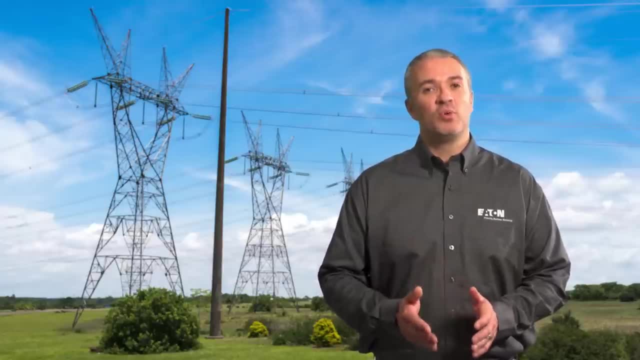 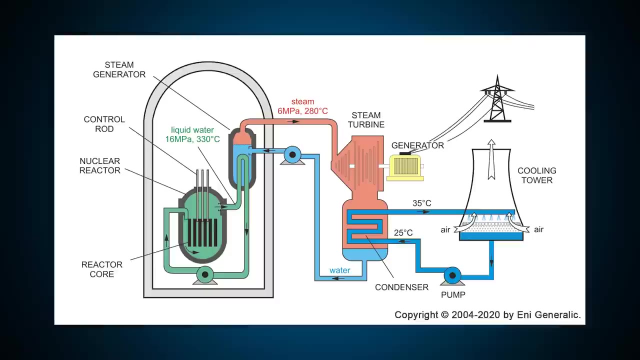 states. it provides around 20 of the electricity used, which is behind natural gas and coal and slightly more than renewables. these plants operate in a similar fashion as fossil fuel plants- by heating water to produce steam, except they don't burn fuels to create heat. nuclear power plants get their heat from a chemical reaction where on the core, 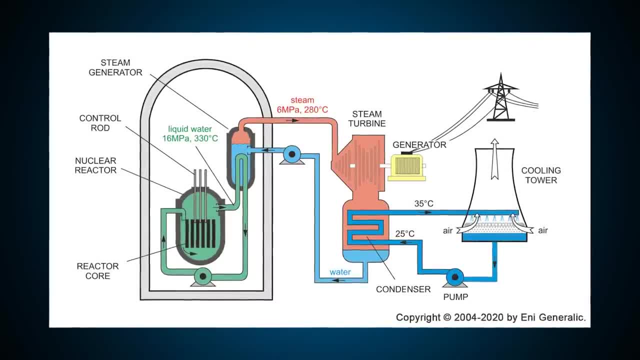 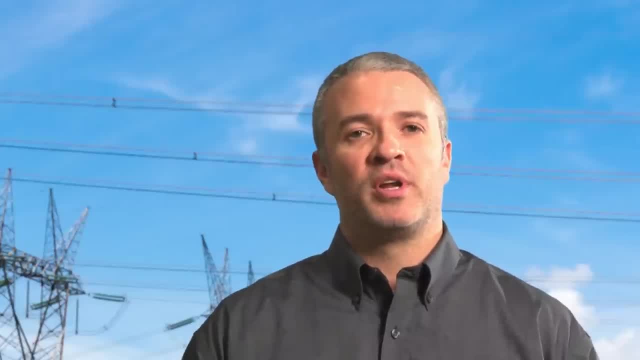 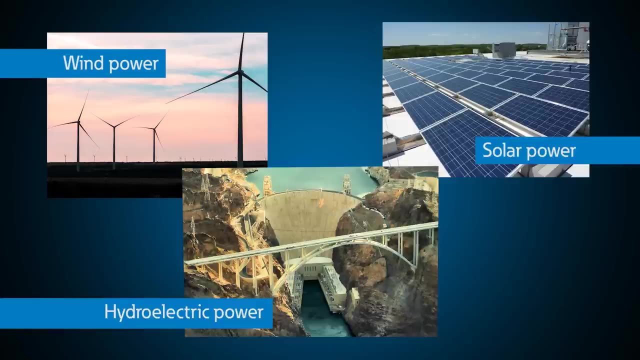 of the nuclear reactor. the fission of uranium atoms releases energy that heats the water to about 520 degrees fahrenheit. renewables are making a large impact with power production in the world and accounting for about a third of the world's generation. the most significant are wind, solar and hydro. hydropower, or hydroelectricity, is by far the largest form of renewable energy and produces about 24 of the world's electricity. in the united states, there are more than 2 000 hydropower plants in operation and account for around seven percent of the total energy. the most. 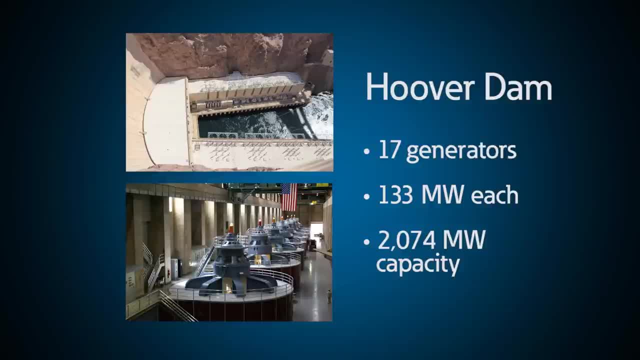 The most well-known hydropower plant in the United States is the Hoover Dam, and it has a total of 17 generators, each able to generate up to 133 megawatts, with a total capacity of 2,074 megawatts. 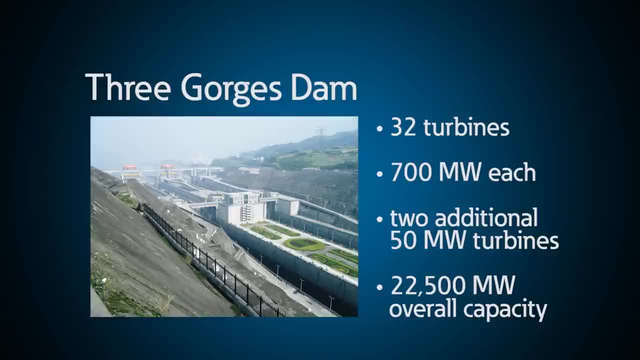 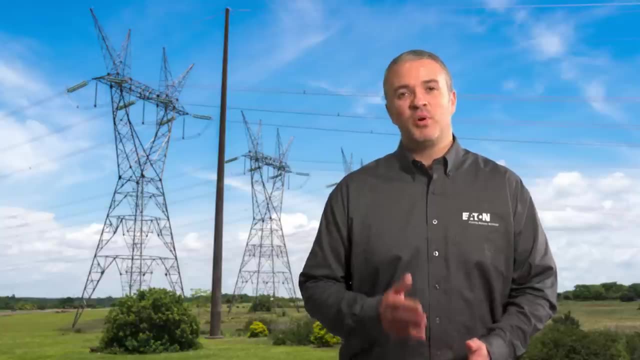 The power plant with the largest available capacity in the world is the Three Gorges Dam in China, which utilizes 32 turbines, each with a capacity of 700 megawatts, and two additional 50 megawatt turbines. That's an overall capacity of 22,500 megawatts. 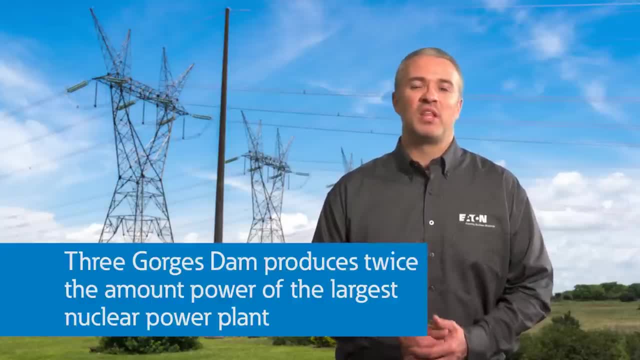 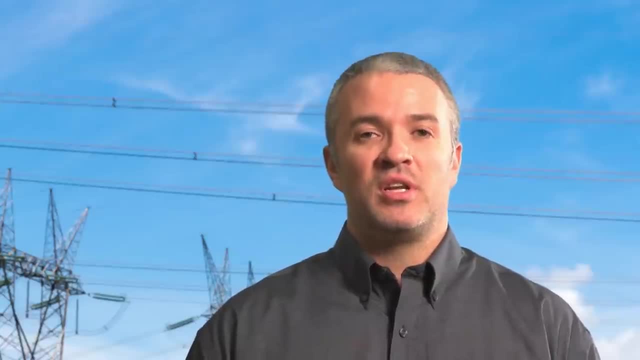 To put that in perspective, that is more than double the amount being produced by the largest nuclear power plant in the world, which is almost 7,500 megawatts. Hydroelectric plants generate electricity like fossil fuels and nuclear power plants, but spin a turbine using the force of water. 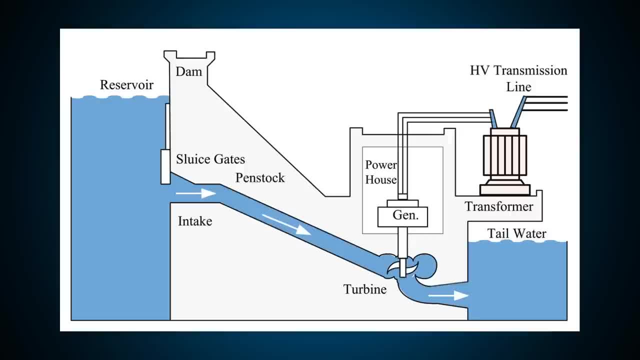 instead of steam. A hydro plant uses the pressure of water created by either a difference of elevation for dams or the force of water in rivers. In either case, the head pressure can be regulated by a control gate. so, when the water flows down a control pipeline called a penstock. 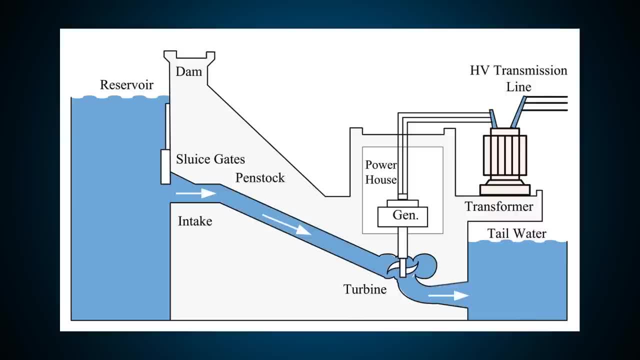 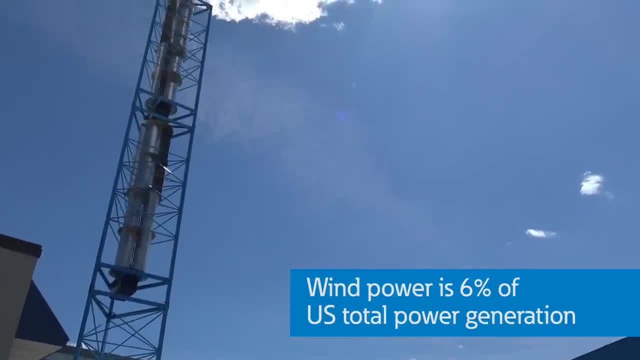 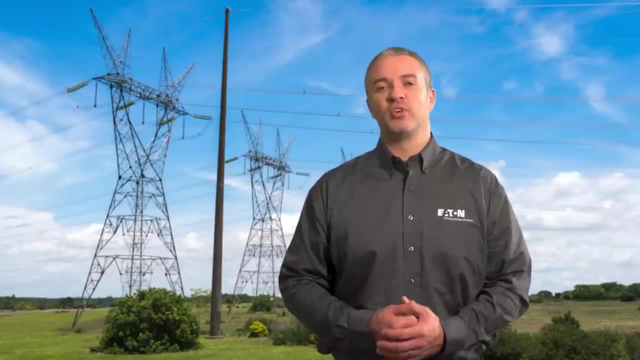 the pressure builds up, spinning a turbine at the bottom and turns the rotor of an AC generator. Wind power is the next highest producing renewable behind hydropower, at 6% of the United States total generation. Wind generation is continuing to rise as more of an effort goes into the production. 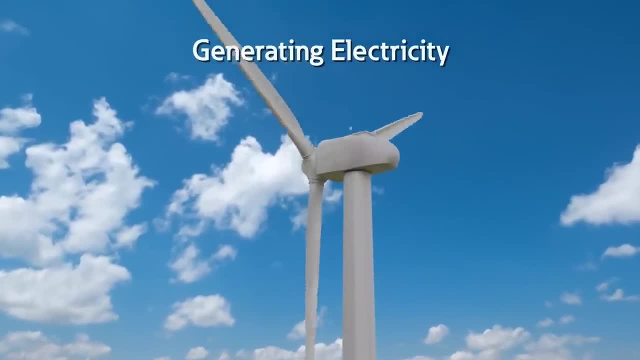 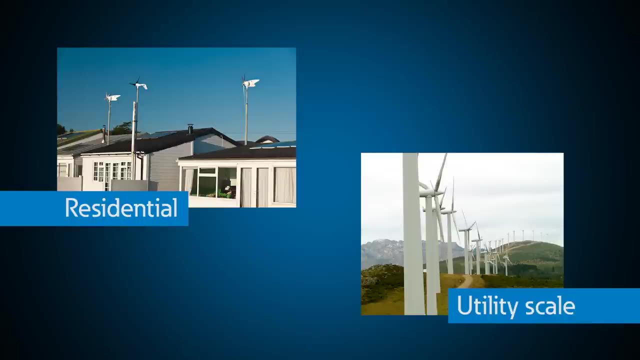 of renewable energy. Wind generation relies on the spinning of a wind turbine that turns the rotor of a generator. This type of generation can be done for individual homes all the way up the utility scale applications that are generally many units connected together as a wind farm. 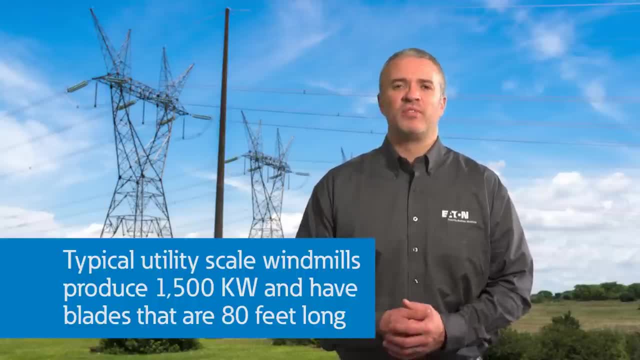 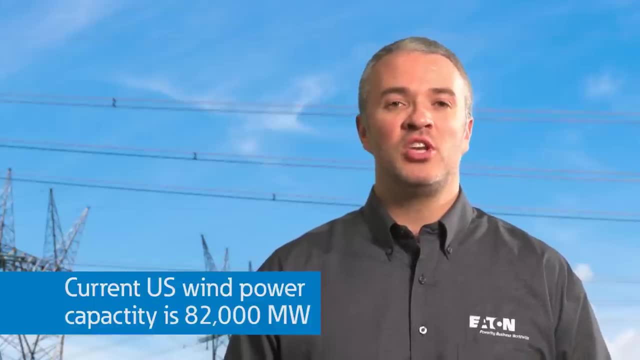 Typically utility scale windmills in the United States produce about 1,500 kilowatts each and have blades that are about 80 feet long. Our current wind power capacity in the US is around 82,000 megawatts, second only to China and the European Union. The US Department of Energy, or DOE, projects the US to have 404,000 megawatts of peak wind power capacity by 2050. That will be enough to fulfill one third of the power demand with all turbines at peak output, if future projections are accurate. 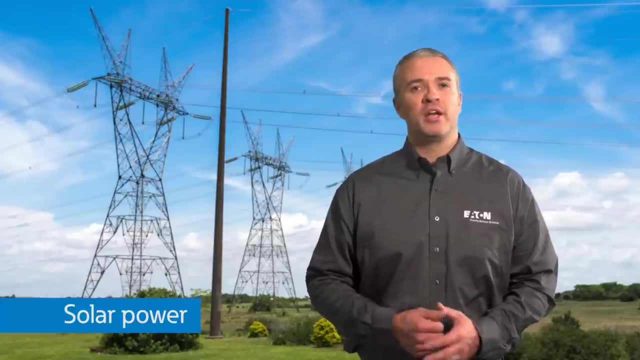 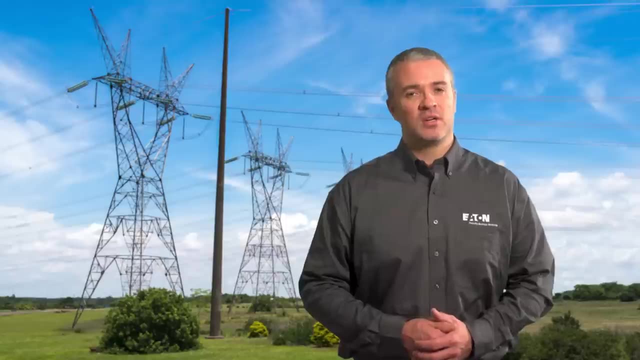 Solar power has been on a steady rise as it becomes more available and a good economic investment. There are lots of incentives in place to promote the growth of solar generation for your home or business. Solar generation is a totally different type of wind power. It's a totally different type of generation. 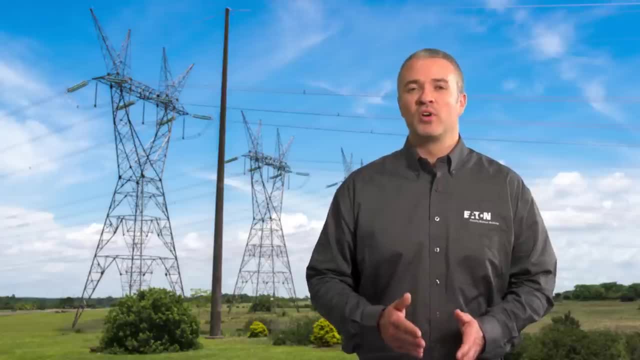 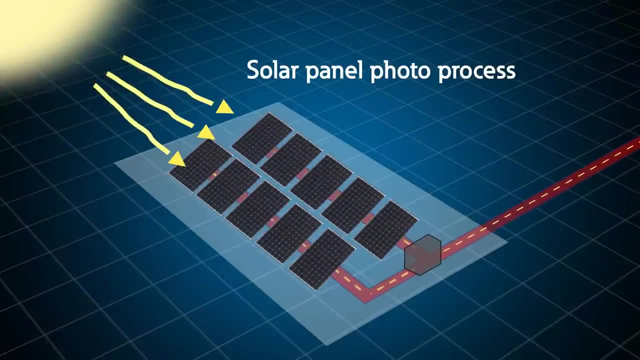 compared to all the others mentioned so far, There is no prime mover or AC generator with solar panels. Solar panels strictly rely on the solar radiation from the sun to be absorbed by photovoltaic panels to produce DC power. The DC power is then converted into AC. 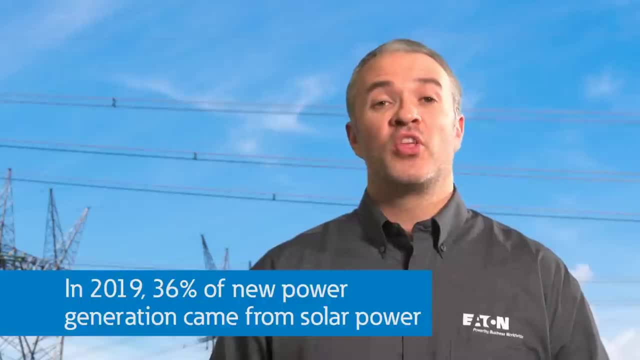 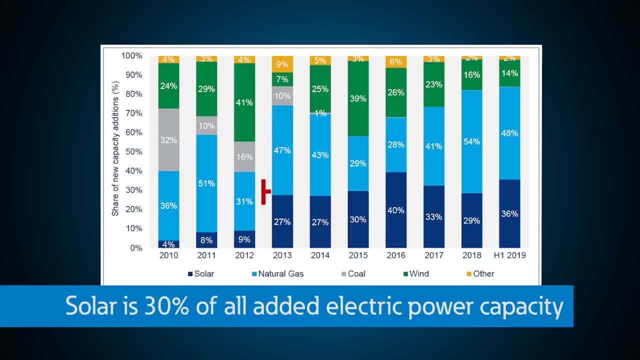 by the use of power electronics inside an inverter. 36% of all new electricity generating capacity additions this past year are actually from solar power. Solar power has been holding quite steady since 2013 by being about 30% of all added electric power capacity. in the United States year over year. Our current solar capacity is 69,000 megawatts, which is on track to double by 2024, adding over 15,000 megawatts each year. Here at the Power Systems Experience Center. 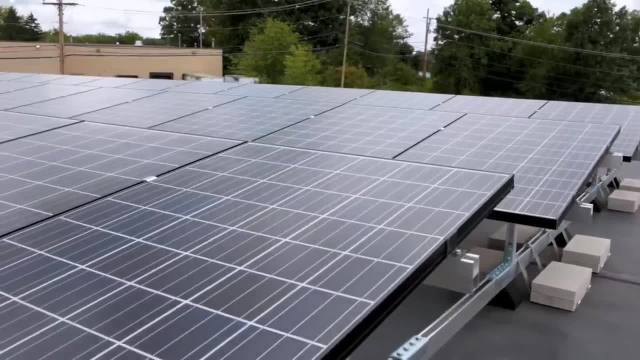 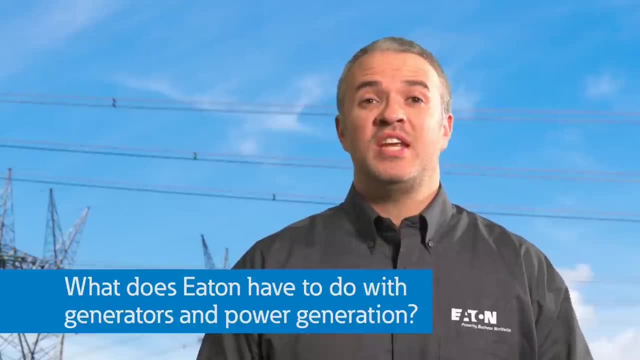 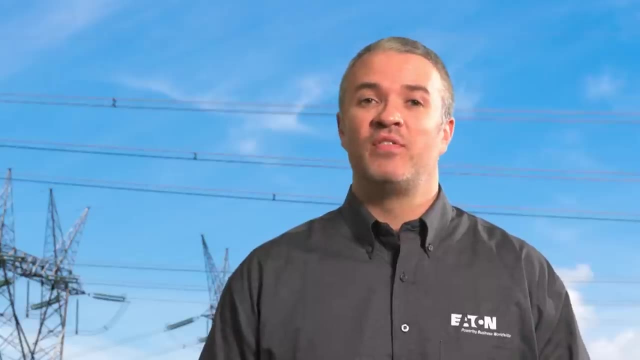 we have a small wind turbine and several different solar installations to illustrate how these alternative energy solutions are viable and can be connected to your grid or microprocessor. So what does Eaton have to do with generators or power generation? Eaton works closely with electric utilities and provides large, medium voltage circuit breakers. 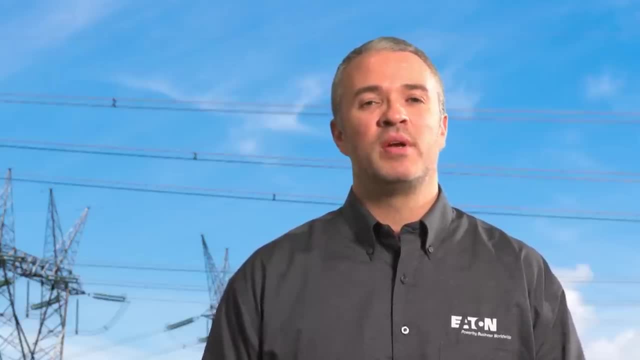 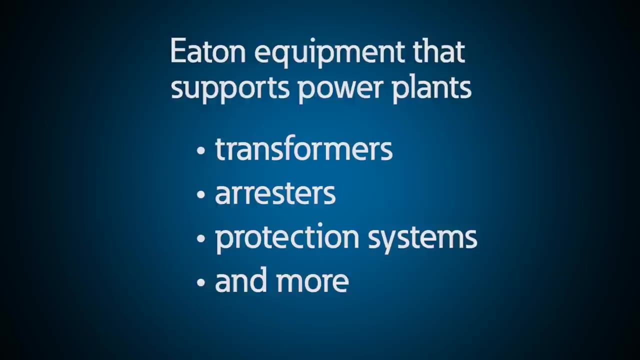 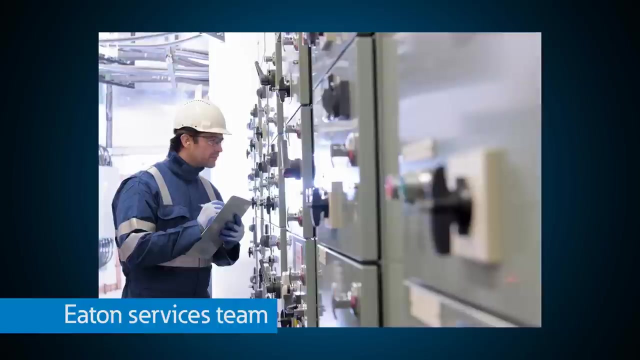 and switchgear for generation stations, as well as electrical equipment to support the operation of these power plants, like transformers, arrestors, protection systems and more. In addition, our services team supports upgrades and reconditioning of existing switchgear and excitation systems. 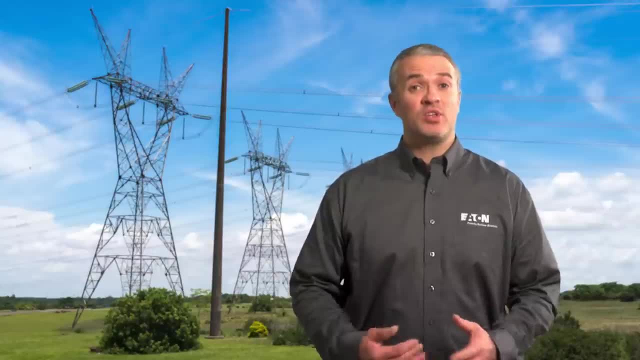 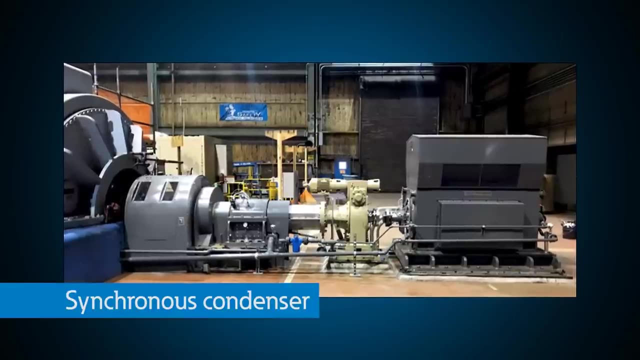 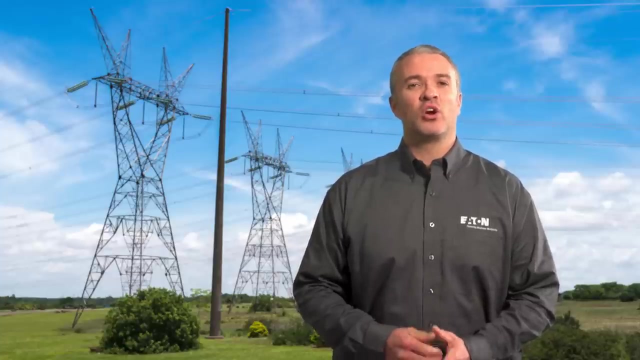 as many of these stations are relatively old, As some utilities are moving away from traditional coal-fired sources. they are converting some generators to synchronous condensers, utilizing much of the same hardware from these generation systems. These large rotating machines can provide or absorb reactive power or VARs to support the voltage. 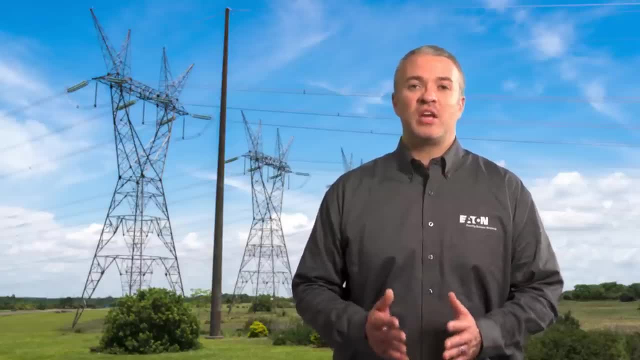 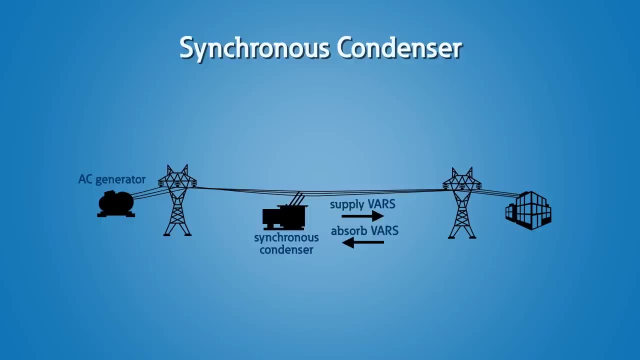 and reactive power requirements of the power grid. A synchronous condenser is a DC-excited synchronous motor whose shaft is not connected to anything but spins freely. This provides stability and voltage control when needed, absorbing VARs when load is lost or providing VARs like a capacitor. 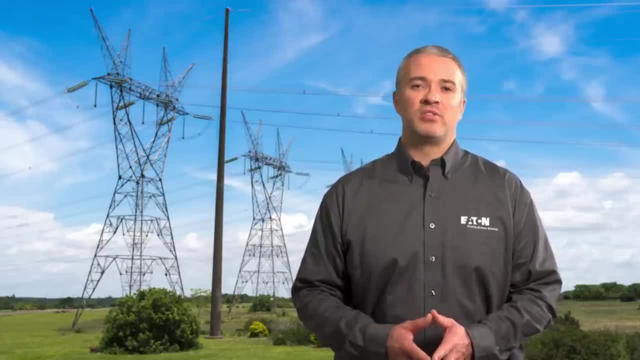 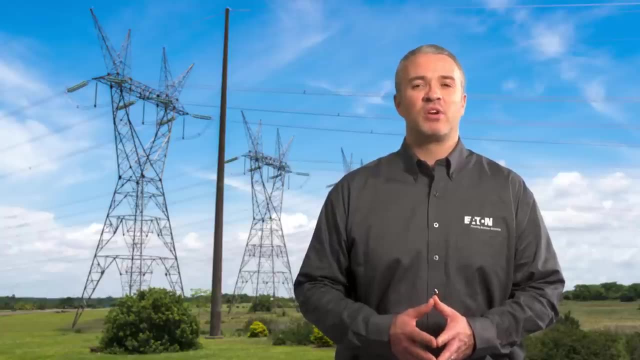 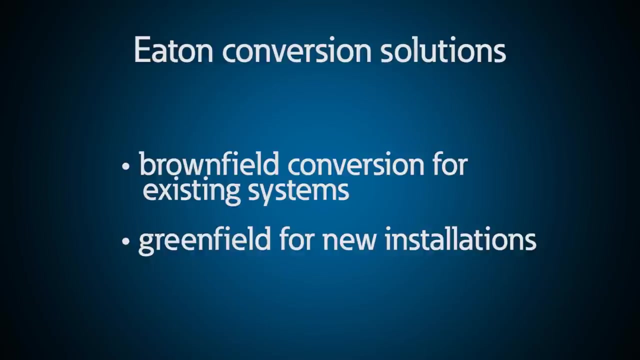 when load is added to the system. Eaton's engineering services group has been very instrumental in several of these upgrades, repurposing the synchronous generators and converting them to synchronous condensers. Eaton offers two solutions: brownfield conversion, converting existing systems, as well as greenfield. 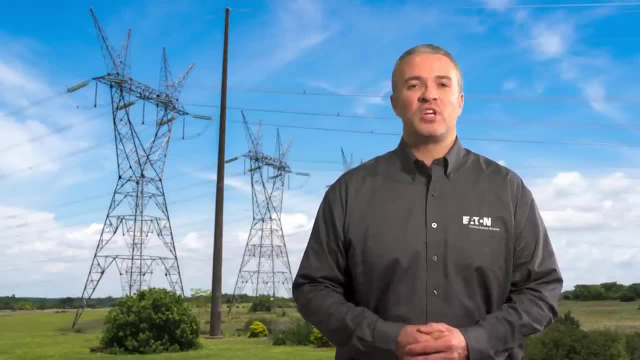 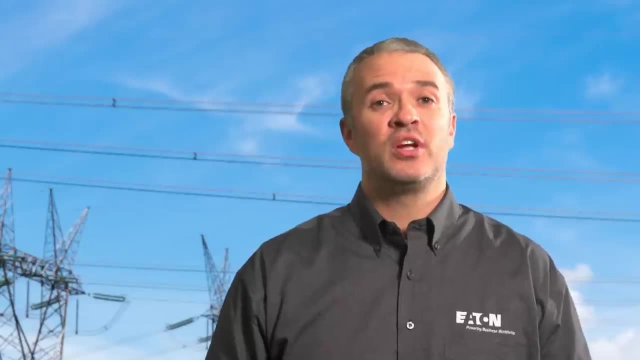 or new installations. These are especially important for systems where wind is a significant power generation source because of the intermittent nature of the wind. In addition to traditional power generation stations, Eaton is heavily involved in the installation and operation of renewable resources, including significant equipment and work. 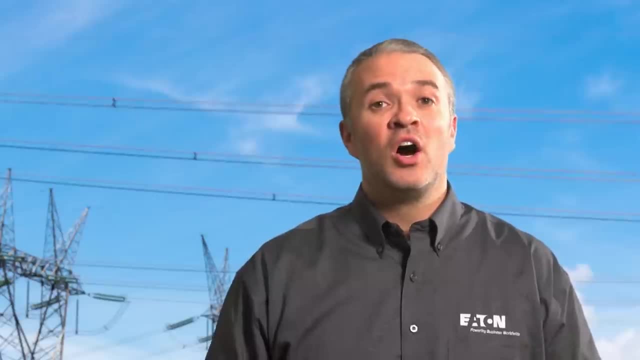 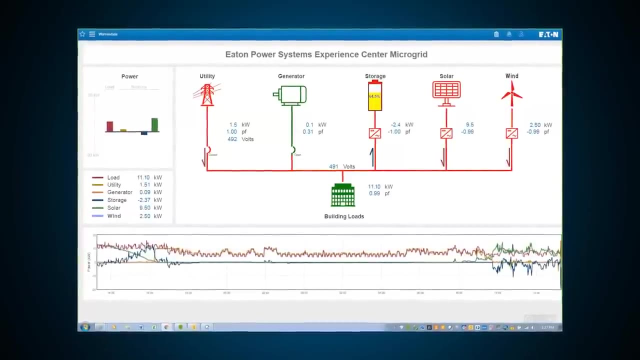 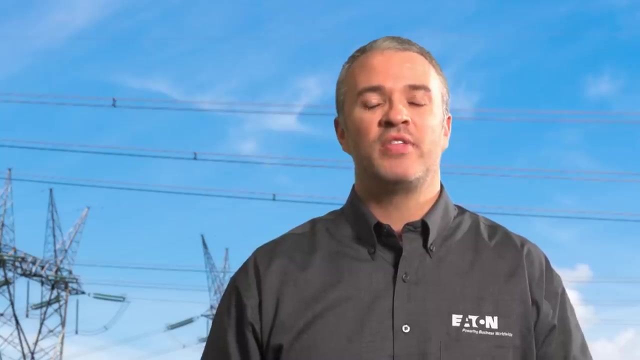 with hydropower and solar installations. Finally, our services team is leading the way in the industry with microgrid solutions tying it all together. Our microgrid energy optimizer can take any generation source or energy storage solution and optimize resiliency and cost, depending on the application. 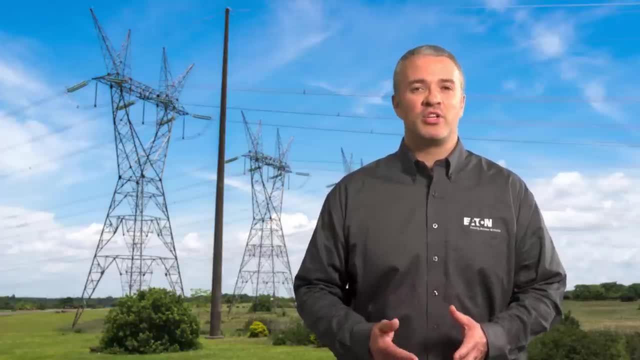 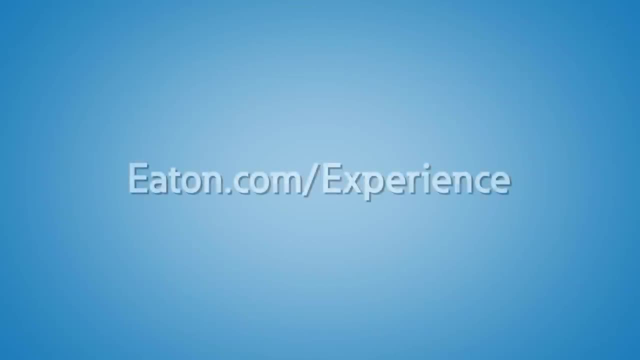 If you want to learn more about different types of power generation, how electricity is distributed after it is generated and how it can be connected to your power system, contact us or your local Eaton representative to schedule a visit to the Power Systems Experience Center today.